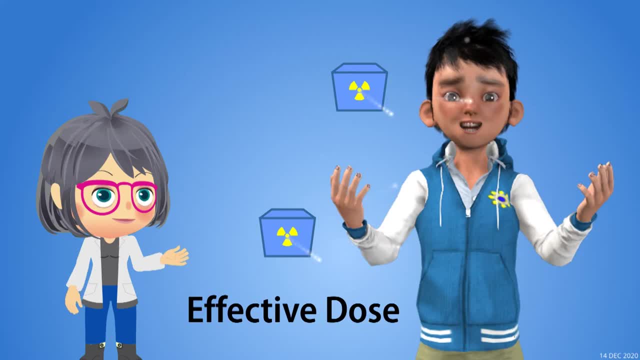 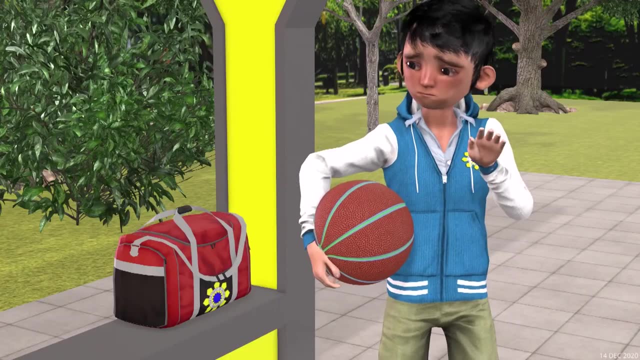 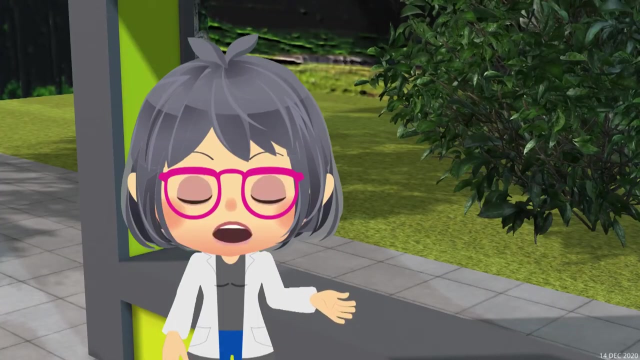 and effective dose. when the type of tissue is considered, Both equivalent dose and effective dose, use Sievert as a unit of measure. Are these units the same ones used for radiation coming from cellular phones? No, These units are only used for ionizing radiation. 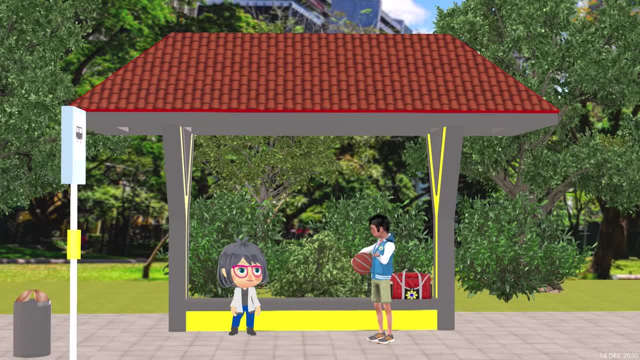 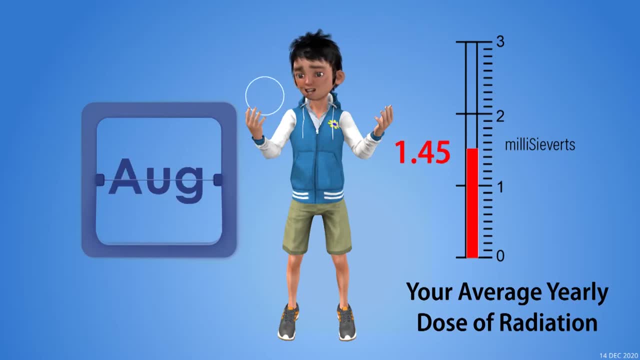 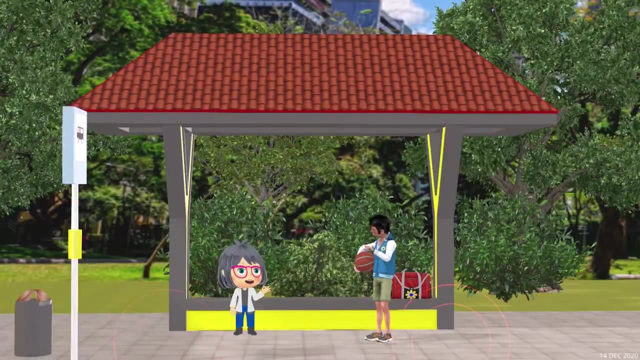 Okay, How much ionizing radiation are we usually exposed to? If coming from natural sources, a person typically receives 2.4 millisieverts of radiation in one year. Even as we stand here, we are exposed to tiny amounts of ionizing radiation from the ground, rocks, buildings and cosmic rays, even from you and me. Just so you can get a clear idea, here's a graph of how much ionizing radiation we receive per unit time, depending on our altitude. And apart from this, there is ionizing radiation that you can get from man-made sources like x-rays and CT scans. 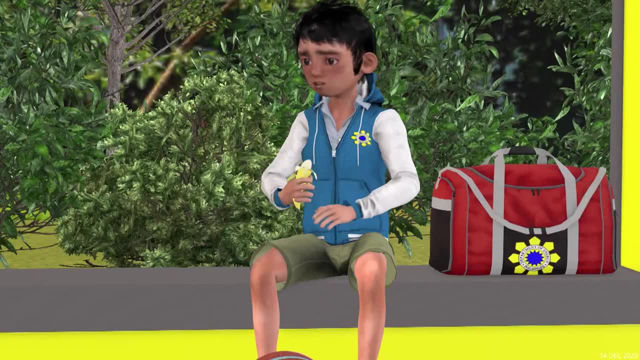 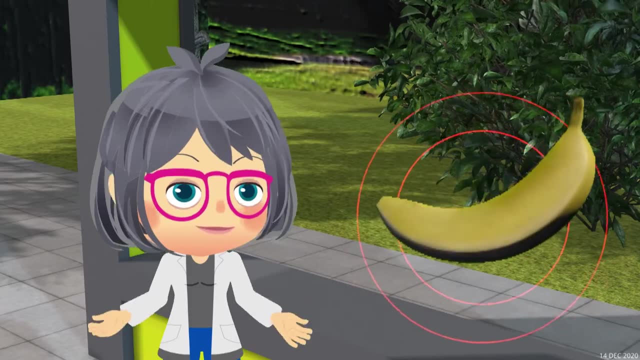 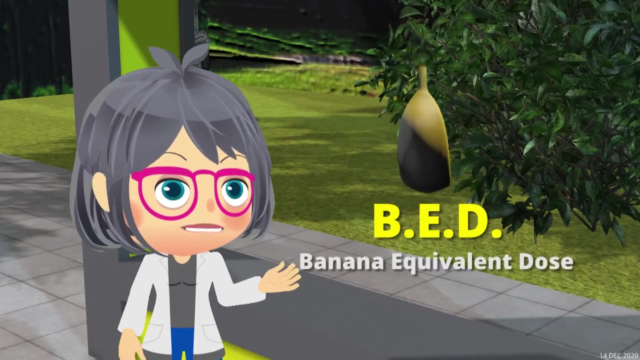 Wow, Radiation is indeed all around us. That's true. In fact, even eating a banana exposes your body to natural radiation. What? Yes, There's even something called BED Banana Equivalent Dose. It's about 0.1 microsieverts. 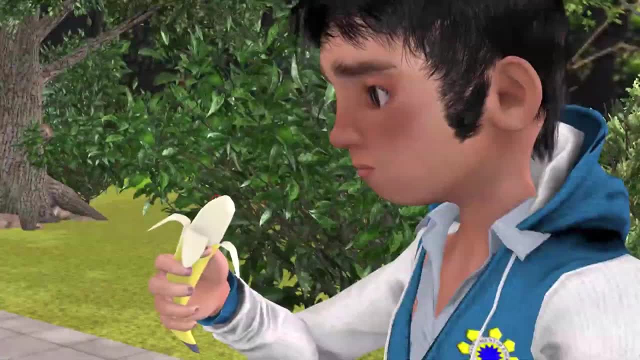 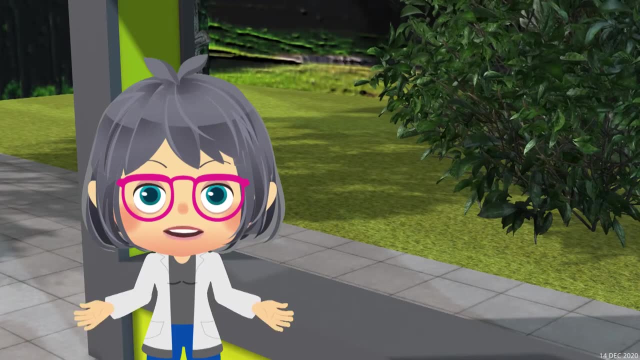 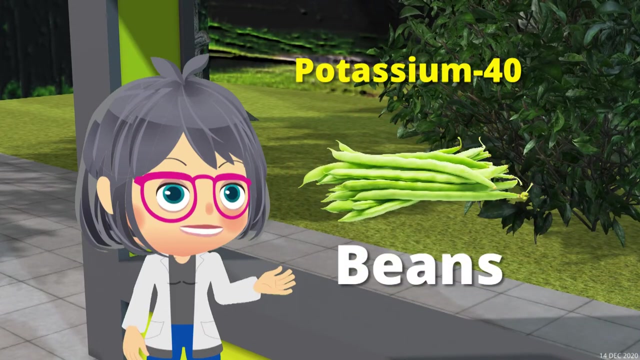 But this is an unofficial unit of measurement. How can a harmless banana even have radiation? You're right for using the word harmless. You see, bananas contain potassium-40.. A radioactive isotope, Potassium-40 also naturally occurs in other foods. 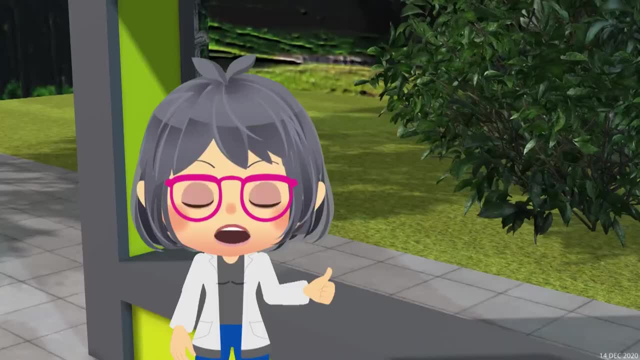 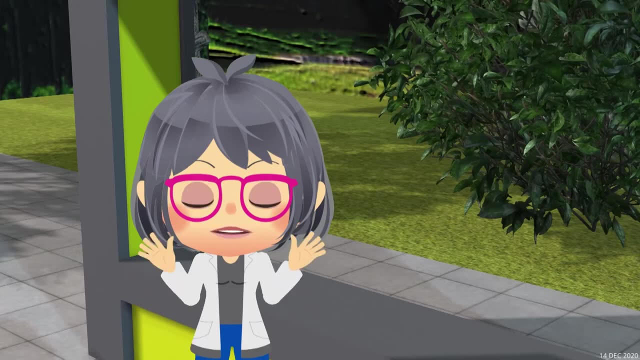 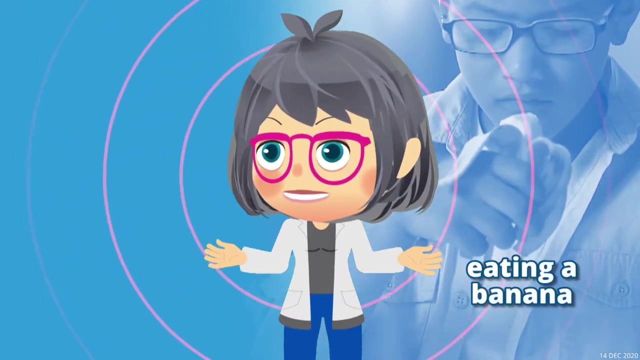 Should I still eat this or not Go ahead? It shouldn't worry you, Because the measure of radiation you get from eating one banana, or even ten in a day, is so small. Let's compare radiation absorbed from eating a banana to radiation absorbed from man-made sources of radiation. 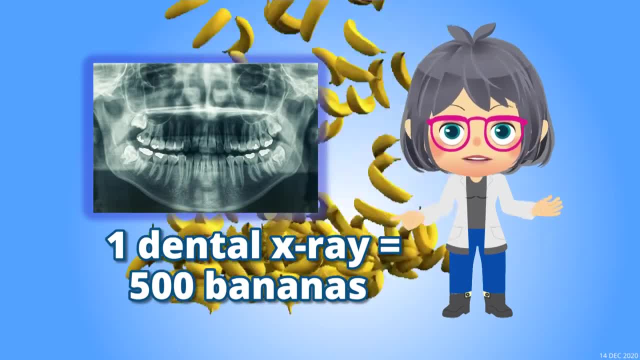 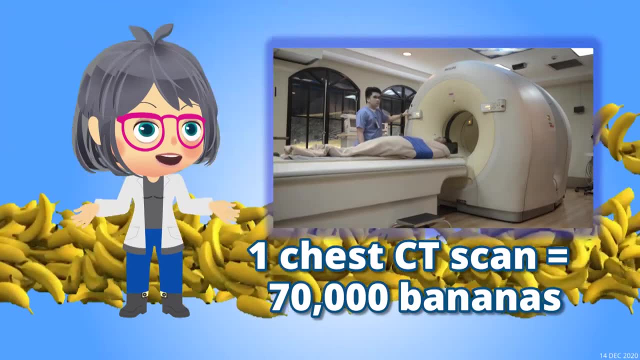 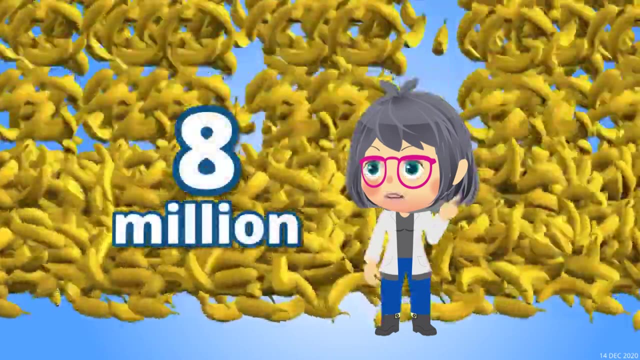 A full dental x-ray is like eating 500 bananas all at one time. One chest CT scan is equivalent to eating 70,000 bananas all in one day. A fatal dose of radiation is equivalent to eating 8 million bananas all in one go. 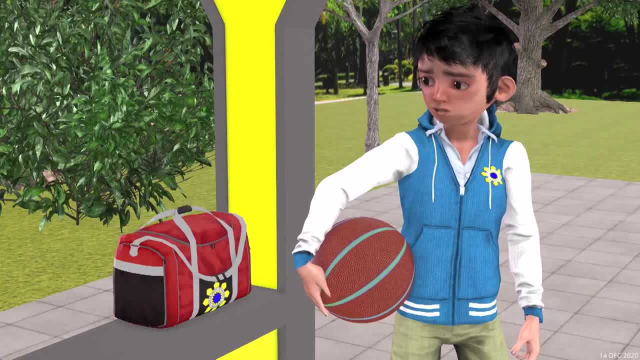 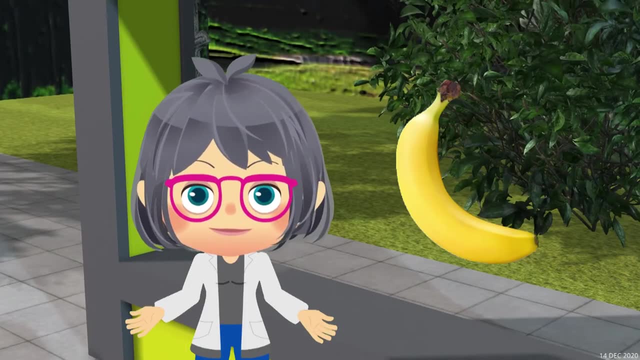 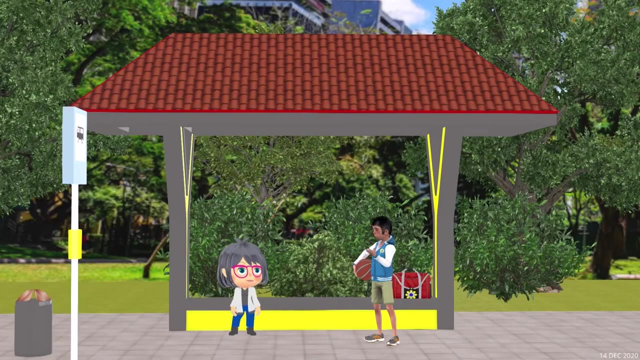 8 million, But that's impossible, Of course. I can't eat that much. That's why eating just one banana is harmless. In fact, some even say eating up to 6 bananas a day is healthy. Okay, so I see how bananas are not really an ideal way of measuring radiation around us. 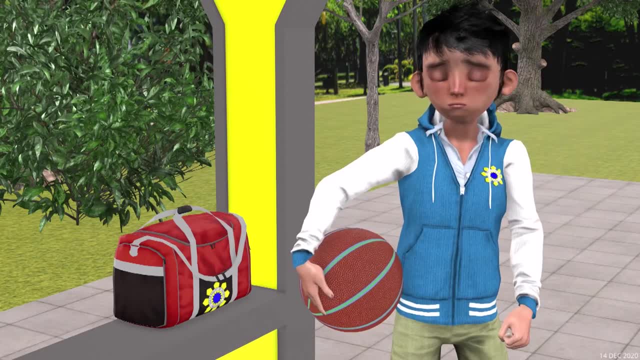 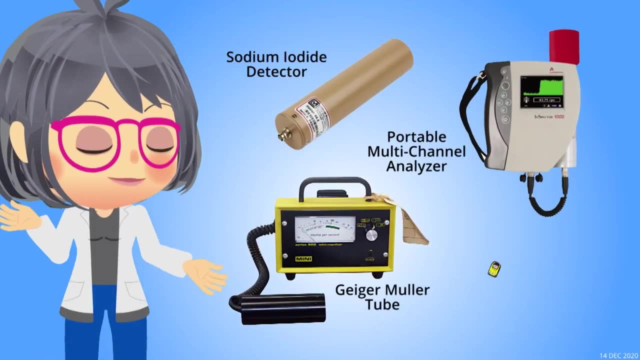 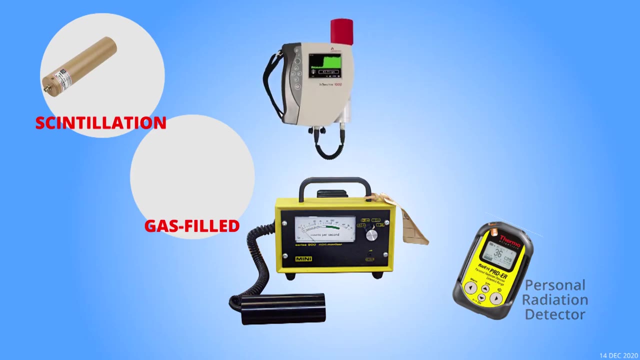 Especially radiation that might be harmful to us. How do we detect it? There are radiation instruments that have been invented and are used to detect and measure the presence of radiation. Since there are several effects of radiation, there are also several mechanisms to detect it. 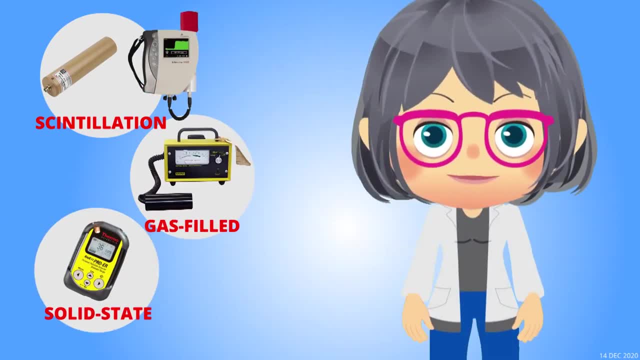 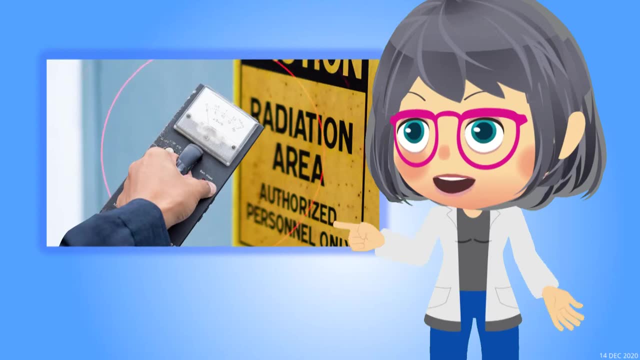 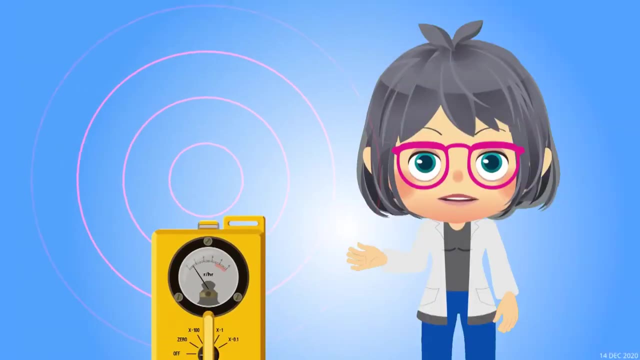 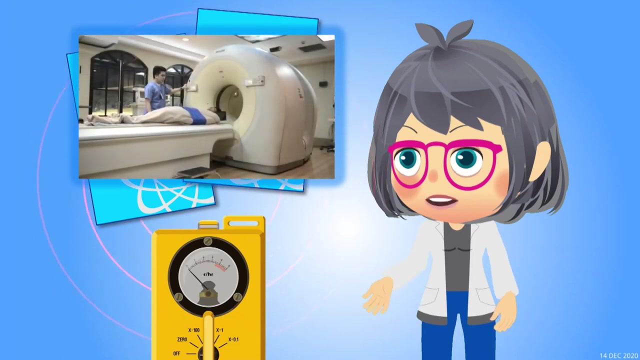 This results to various types of radiation detectors. These serve different purposes. Apart from being radiation monitoring instruments, some are also used for personal dosimetry Cool. Having the means to measure radiation properly makes it easier to implement radiation protection standards that are crucial in nuclear science and technology-related industries. 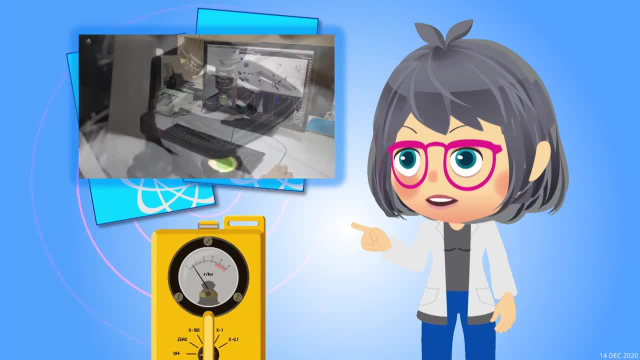 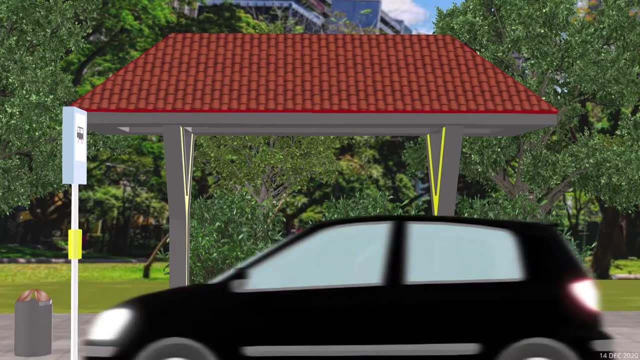 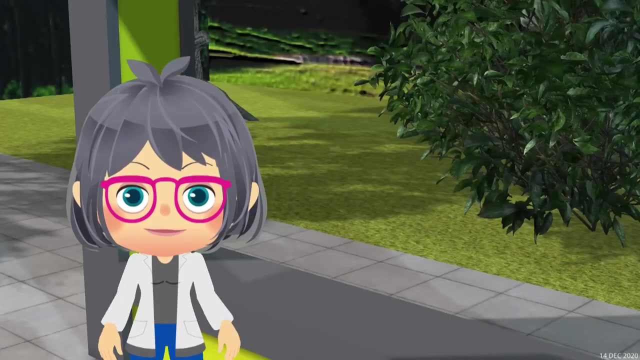 There are also many other industries that have been utilizing the benefits of radiation for scientific gain, as well as for diagnosing and curing some diseases. Wow, so there are rules governing the use of radioactive sources. Not anyone can just go inside nuclear facilities, right? 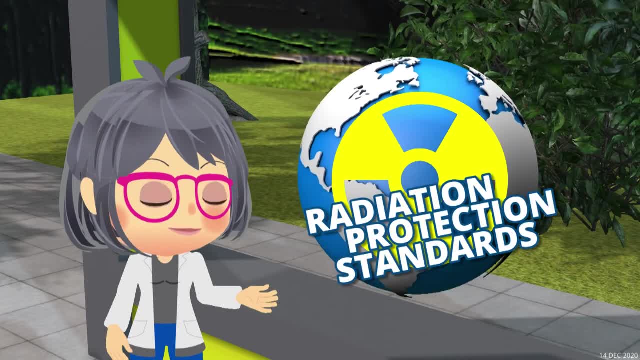 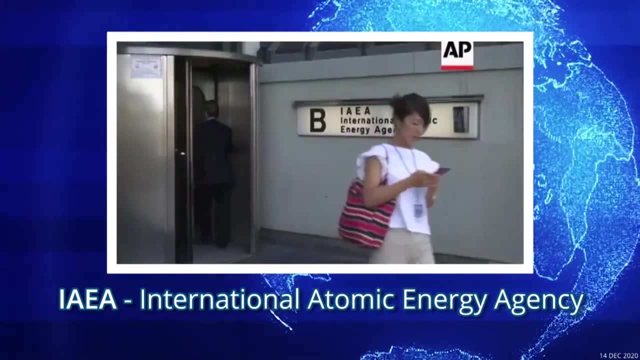 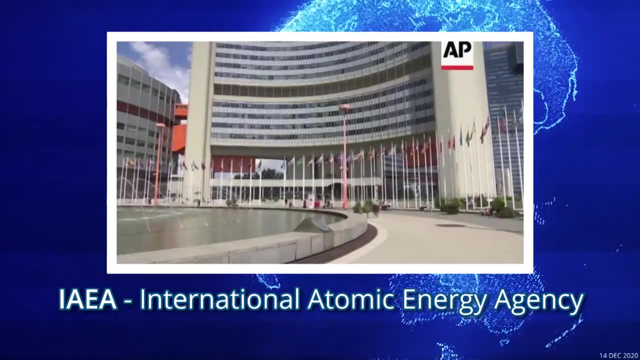 Of course not. Radiation protection standards are implemented worldwide. The International Atomic Energy Agency, or IAEA, works hand-in-hand with its member states, like the Philippines, and other international organizations in order to establish and implement safety standards. I feel quite safer now. 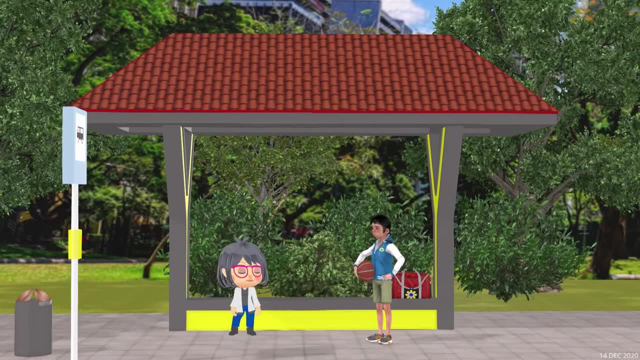 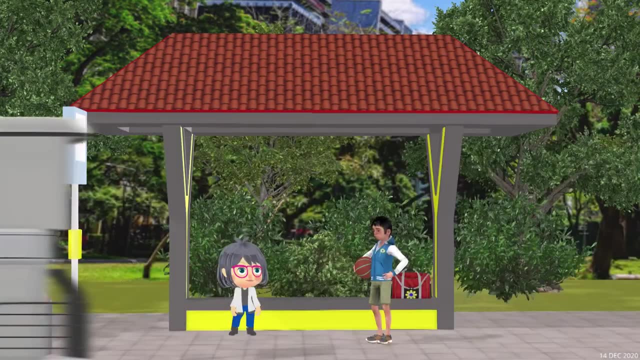 But if radiation is used in so many aspects of our lives, like x-rays and CT scans, and we encounter it every day from natural sources and our body does absorb some of it, does that mean these accumulate in our bodies through many years? Aren't we all supposed to be highly radioactive by now? I mean, where does all this radioactivity go? No, our bodies do not accumulate radiation. You do not become radioactive just because you're exposed to radiation. As for radioactive sources, they do not stay radioactive forever. 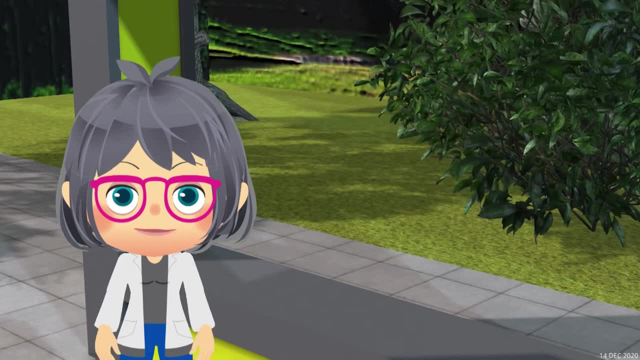 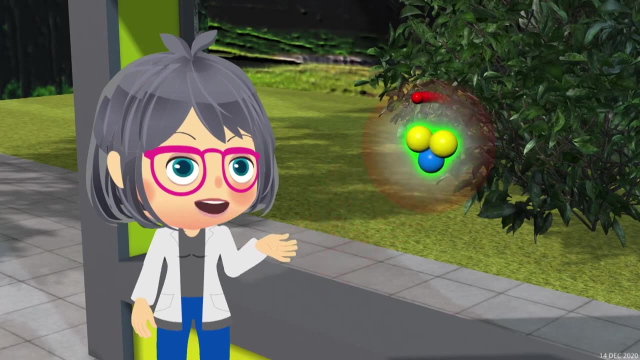 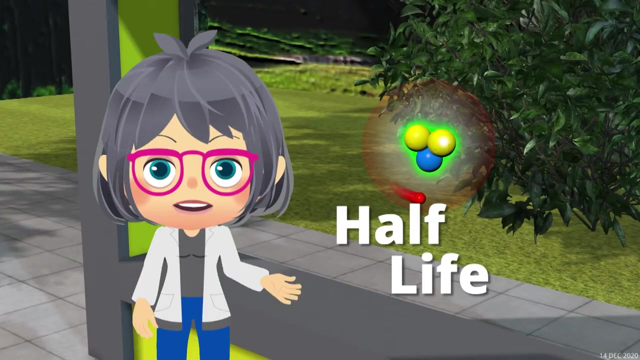 Radioactivity goes away on its own, naturally. What? How? Remember how radiation in itself is a process of nuclear decay. Thankfully, any radioactive substance has what we call a half-life, A half-life. Yes, All radioactive substances have a half-life.